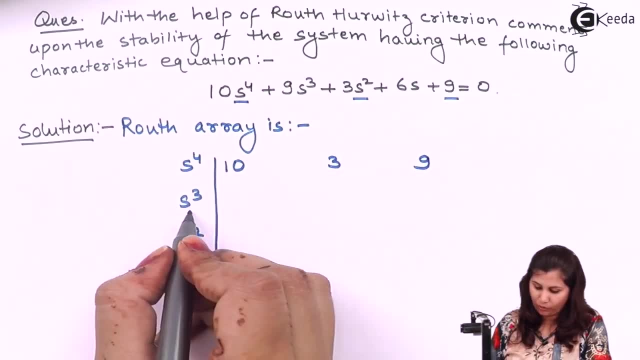 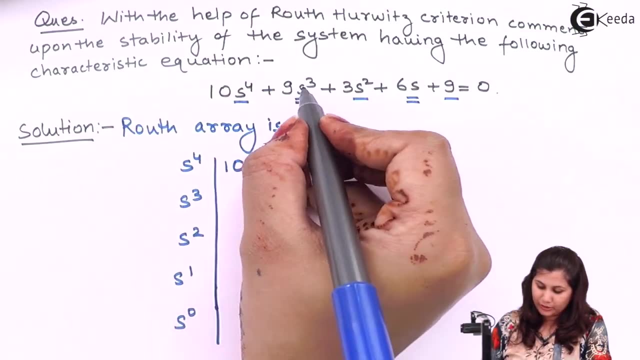 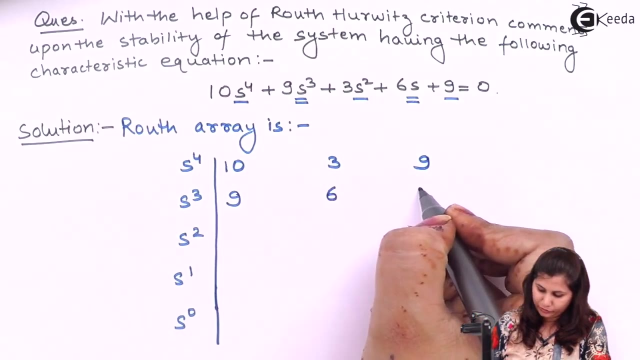 Next, we have s to the power 3.. So we have odd terms. So we will write the coefficient of s cube s to the power 0.. So we have odd terms. power 1: okay. so s cube coefficient is 9, s coefficient is 6 and below this we will write. 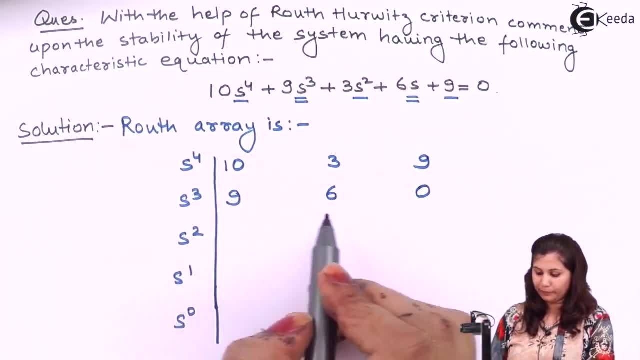 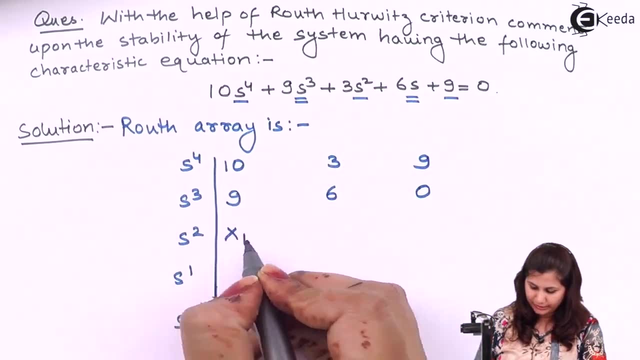 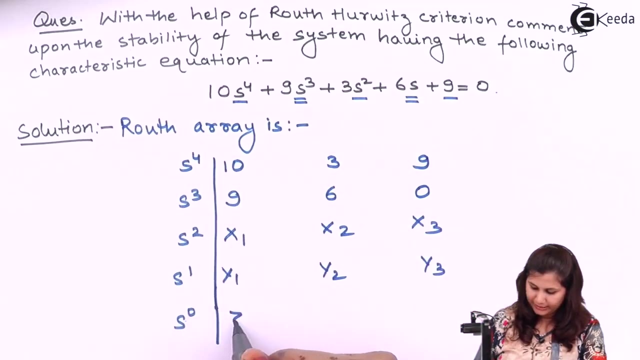 0. if there is no coefficient here, then we will. to complete the array, we will write here: 0. now s square. it will be x1, x2, x3, y1, y2, y3 and z1, z2, z3. the remaining elements we have to find out. 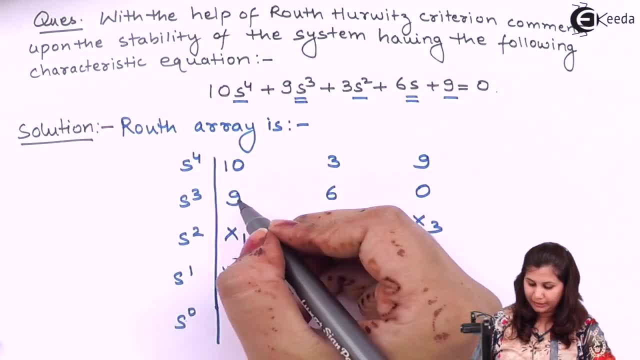 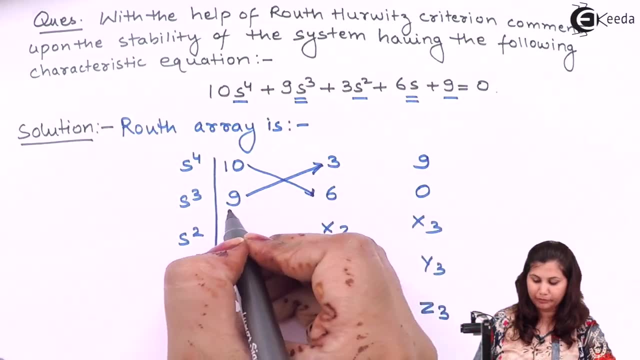 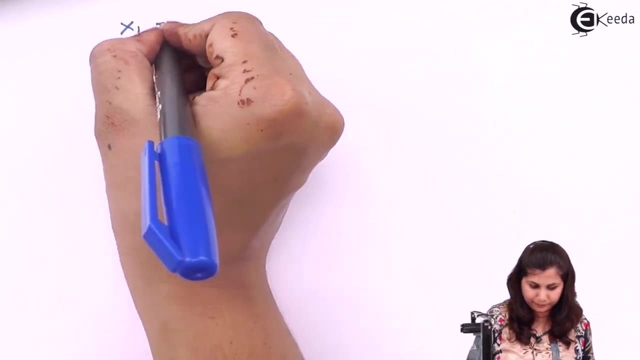 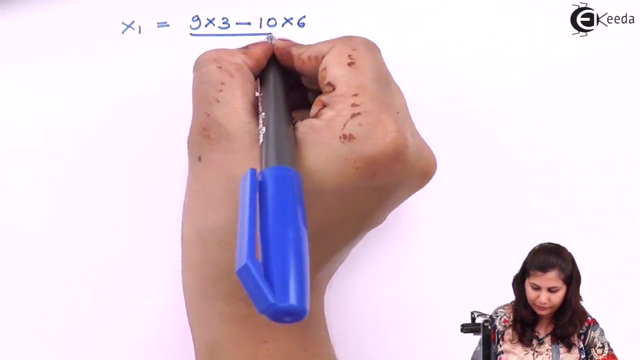 so x1. it will be given by the multiplication of 9 into 3 minus 10 into 6 and divided by 9. okay, so x1 is 9. what 9 into 3 minus 10 into 6, divided by 9.. So it will be equal to 9 threesome. 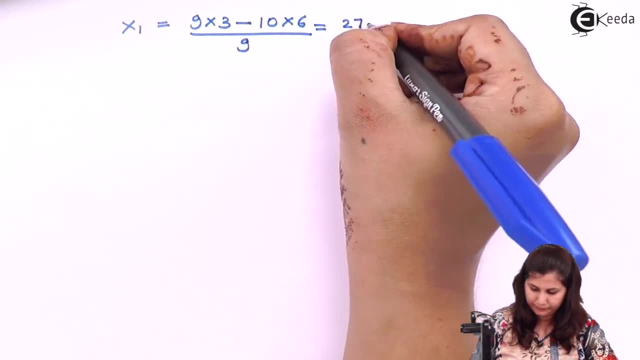 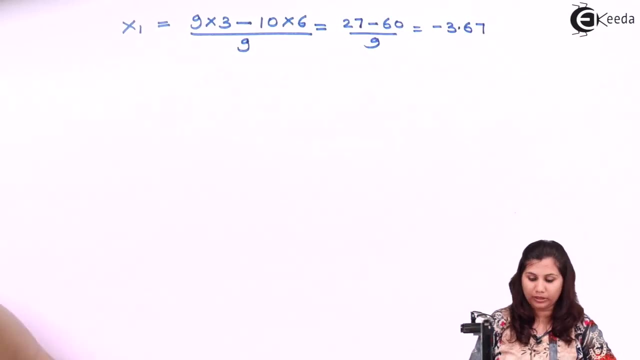 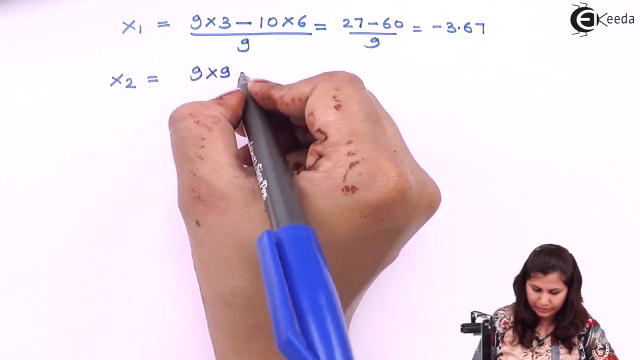 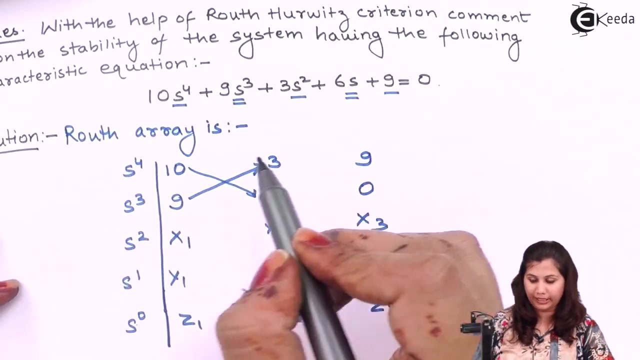 It will be minus 3.67.. Okay, Then we have x2.. So it will be 9 into 9, minus 10 into 0.. How we can find out it? 9 multiplied with 9.. So 9 into 9 minus 10 into 0, divided by 9.. 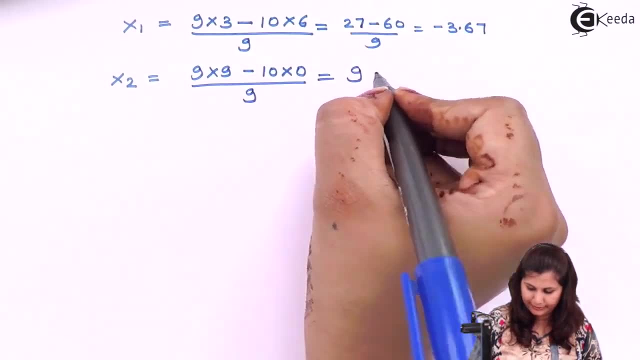 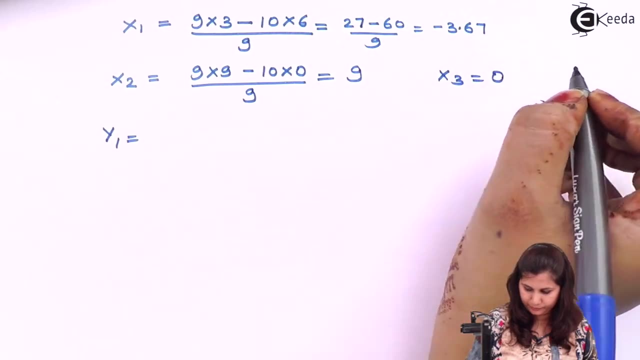 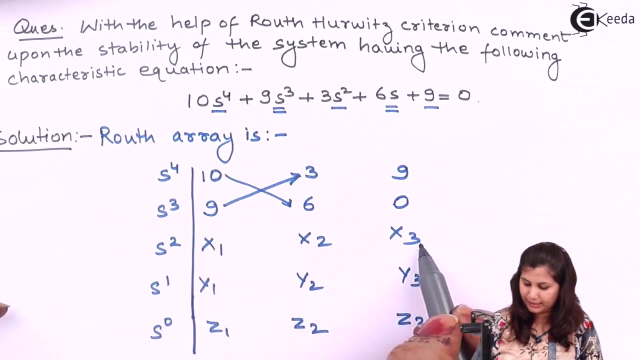 So it will be 9.. Then we have y1.. x3 will be equals to 0.. Okay, Because we are not having the third again. on other terms, we are not having, So this x3 will be equals to 0.. Now y1.. y1 can. 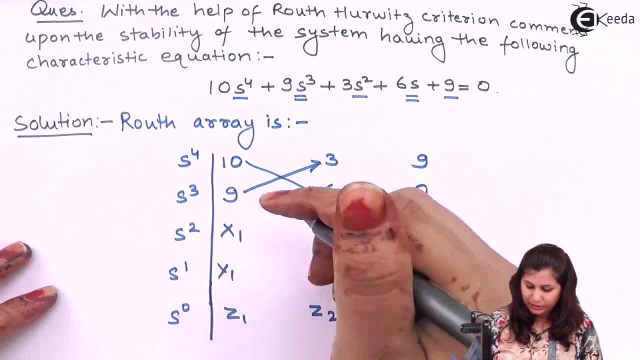 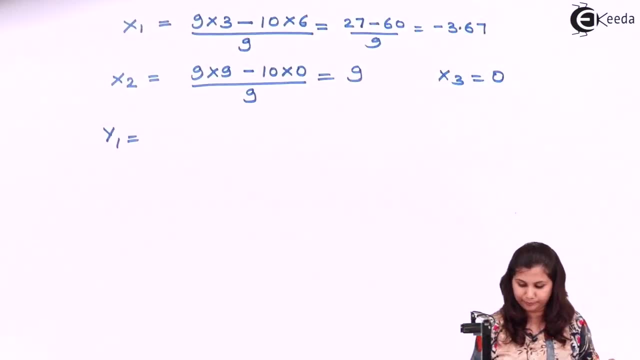 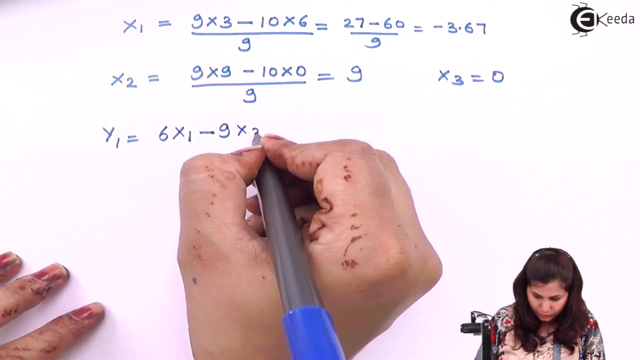 be determined by having this x1. x1 multiplied with 6. Then 9 into x2. Divided by x1. So it will be 6x1 minus 9x2 upon x1. Putting the value of x1 here, we will have: 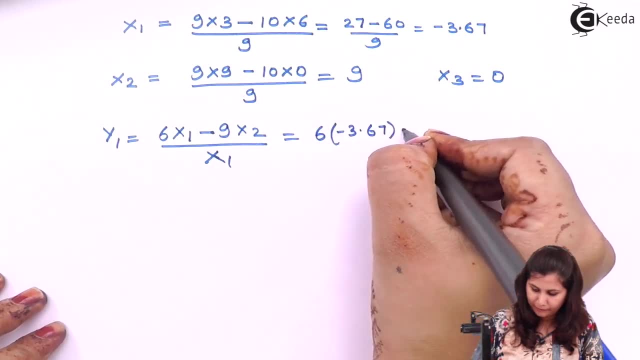 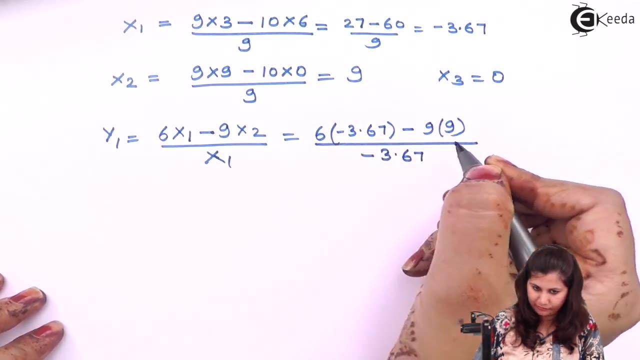 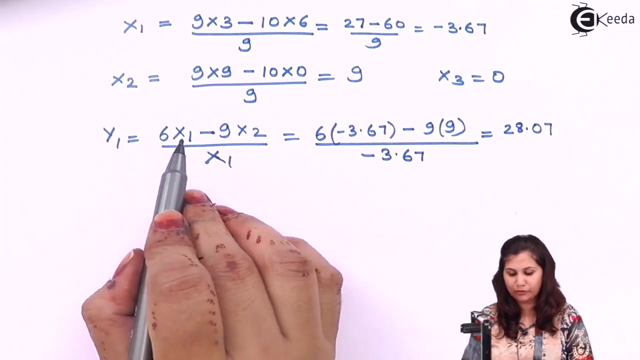 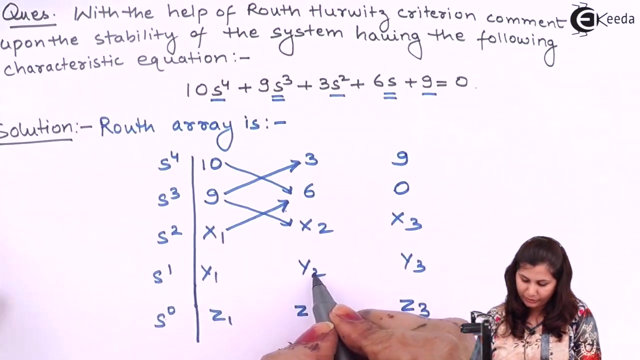 6 into minus 3.67, minus 9 into 9 upon x1 is what Minus 3.67.. So when we solve this we will get 7.. Just put the value of x1, x2 in this equation. Now we have y2.. How we can calculate y2? y2 will. 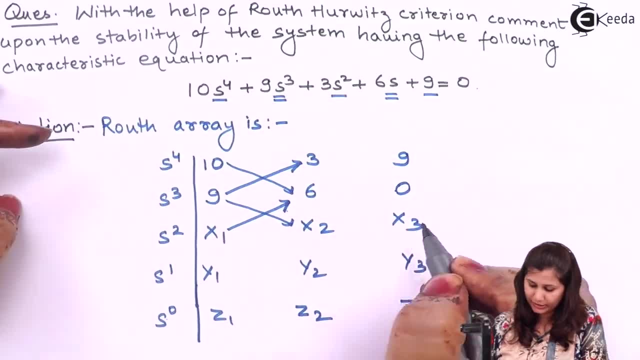 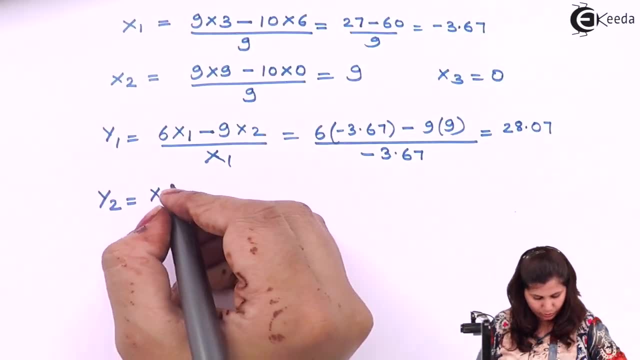 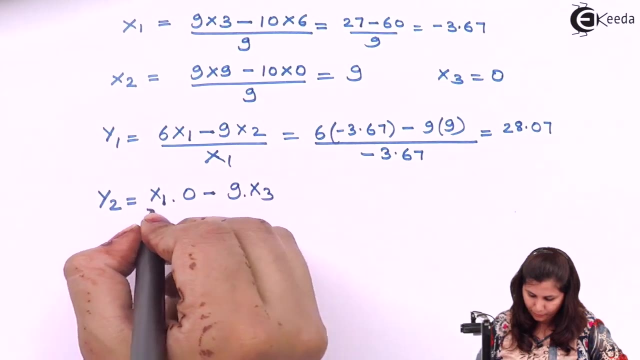 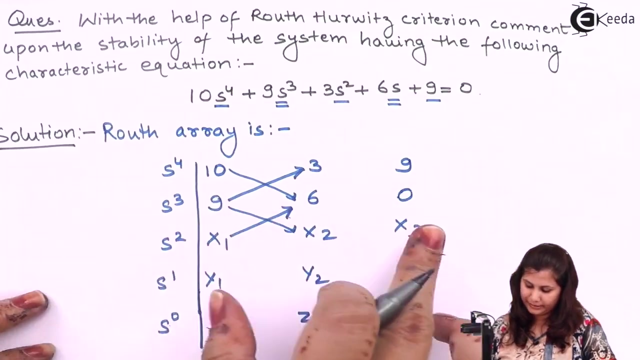 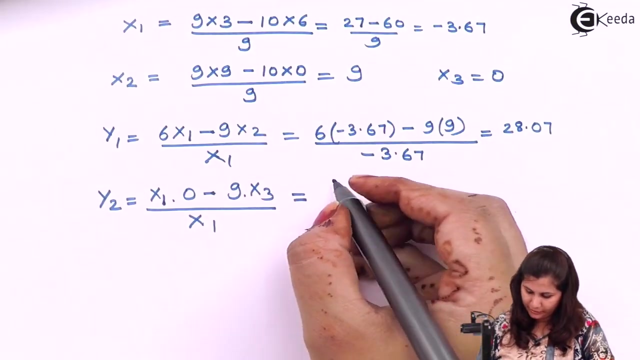 be y1 into x3.. x1 into y3 divided by y1.. So it will be x1 into this, 0 minus 9 into x3 upon x1.. x1 into 0 minus 9 into x3 divided by x1 will be y2.. So putting the value of x1 minus 3.67 into 0, 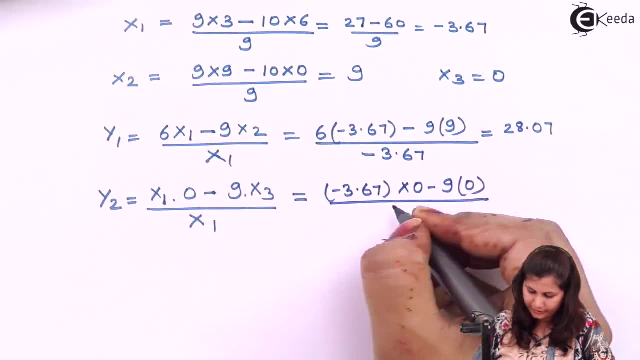 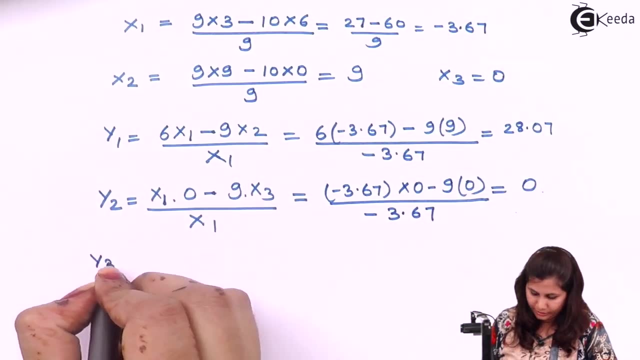 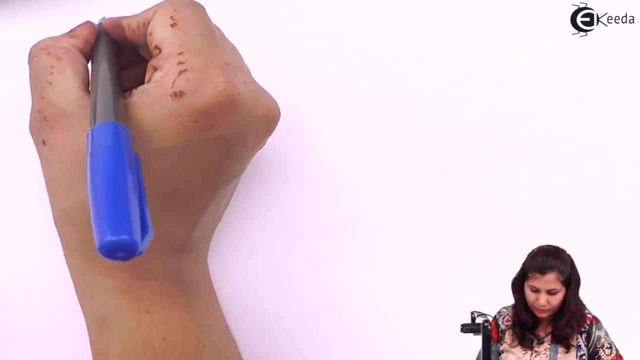 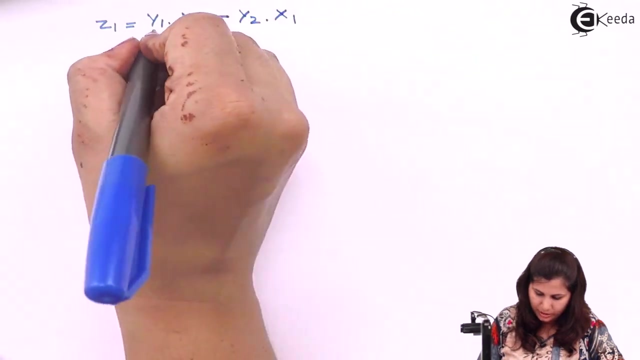 minus 9.. x3 is what 0 divided by x1, that is minus 3.67.. So it will be 0.. y3, it is 0.. Then we have z1.. z1 will be what y1 dot x2 minus y2 dot x1 upon y1.. In the array you can see what it will be. 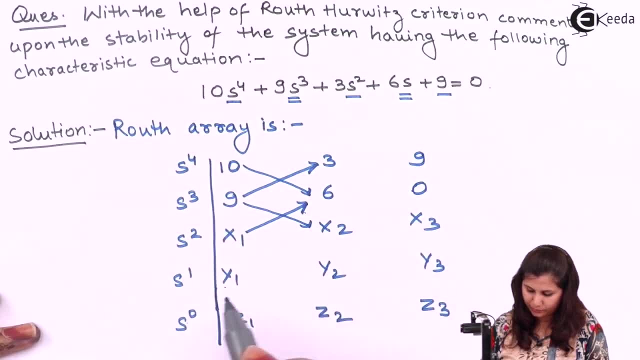 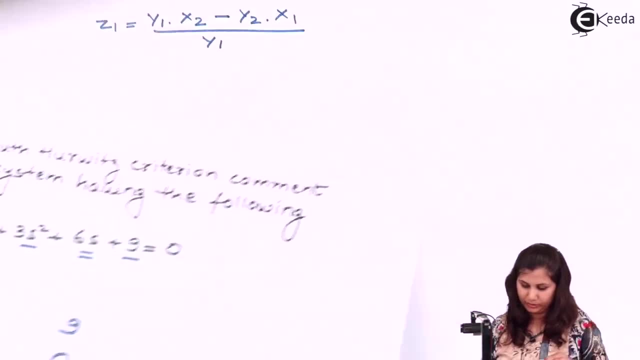 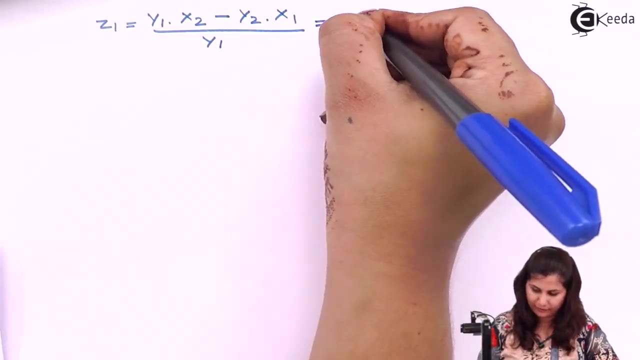 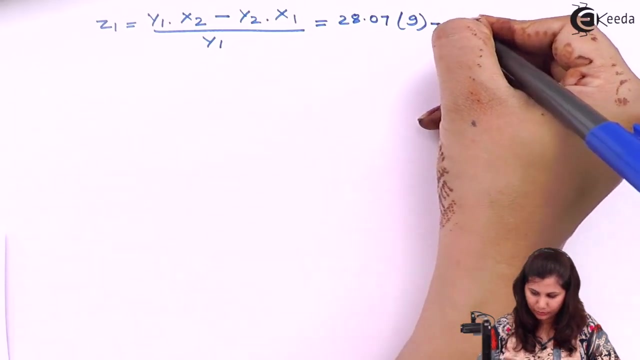 y1 into x2 minus y2, x1 divided by y1.. And what is z2?? y1, x3 minus x1, y3 upon y1. Substitute its value. y1 is what We have obtained 28.07.. So 28.07 x2 is what 9 minus y2 is what 0.. x1 is minus 3.67 and divided. 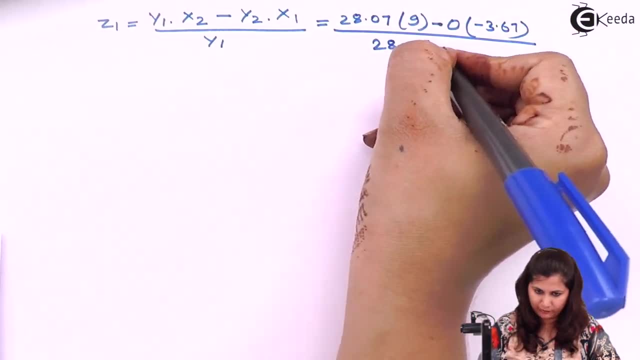 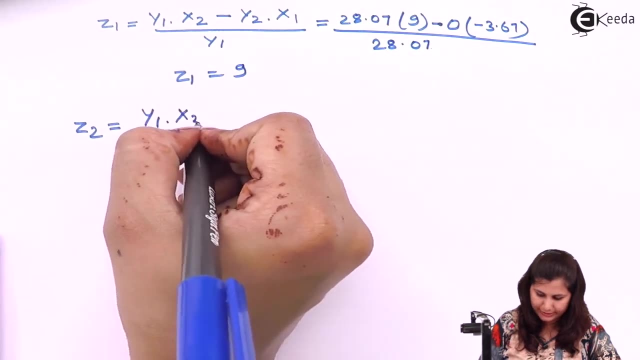 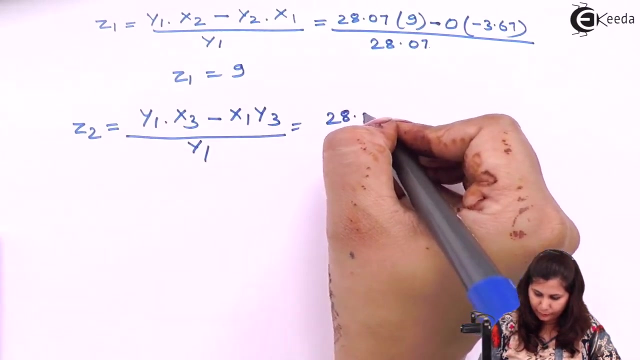 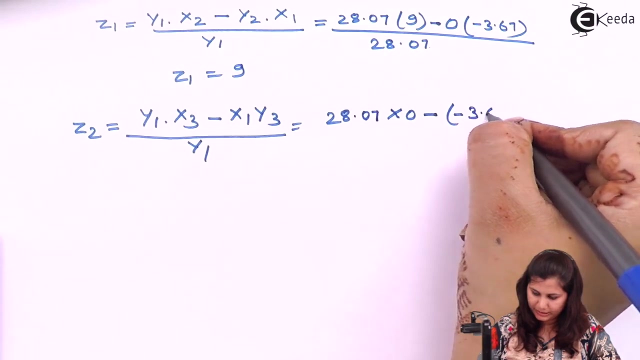 by y1.. y1 is 28.07.. So z1 will be 9.. z2 it is y1 dot x3 minus x1, y3 upon y1.. Putting the values we have 28.07 into 0 minus, we have: x1 is minus 3.67 and y3 is what 0 divided by y1. y1 is: 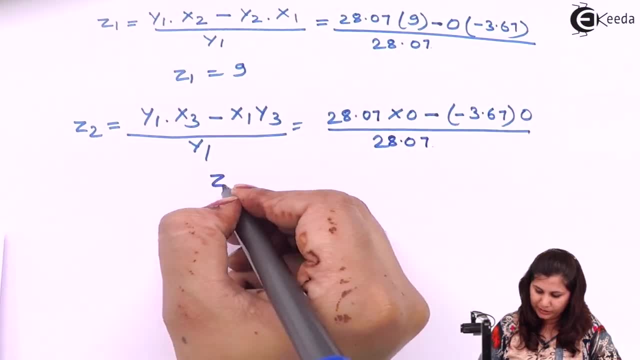 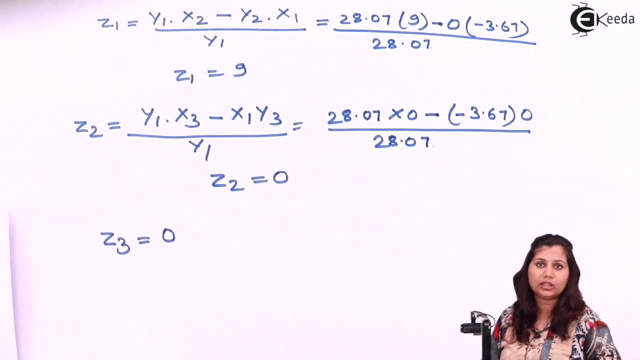 what 28.07.. So z2 will be equals to 0. Now z3 it will be 0. So we have calculated all the coefficients, or all the elements of the root array. So form the root array what it is. 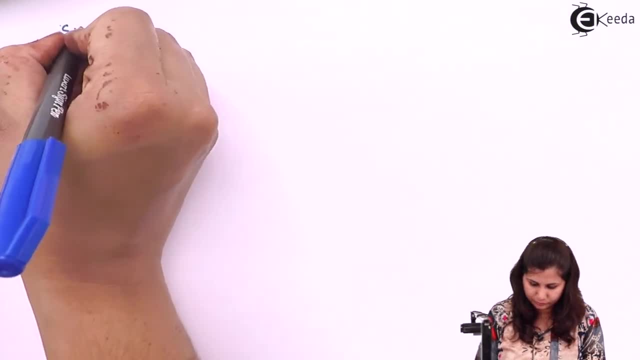 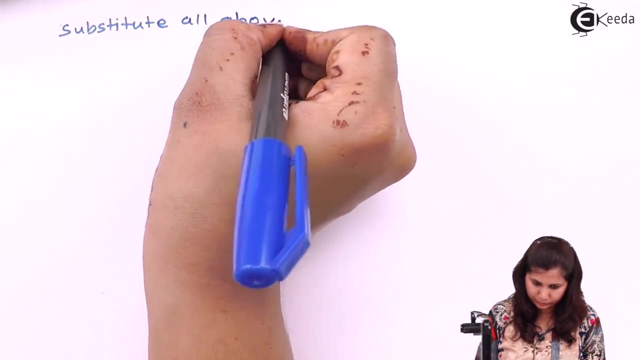 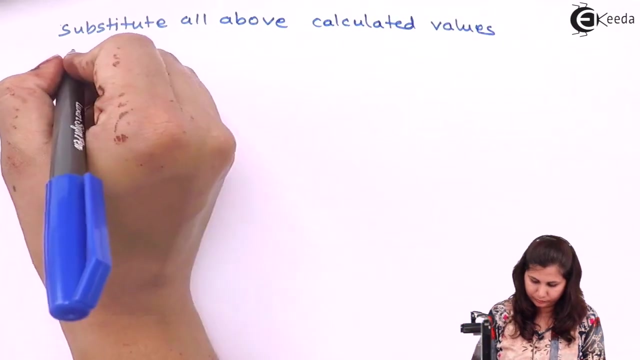 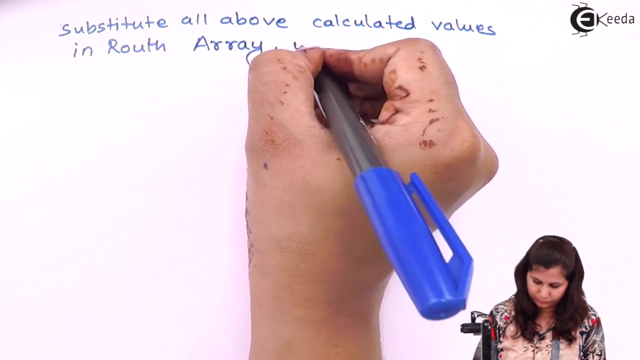 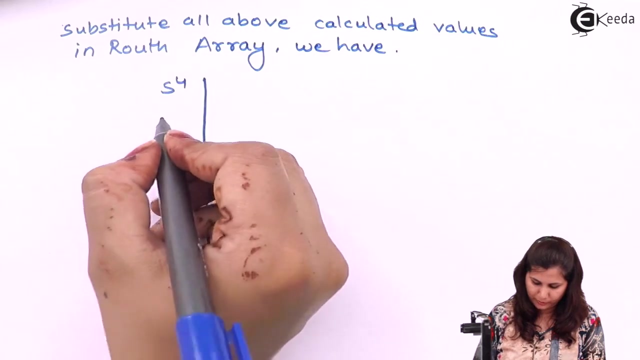 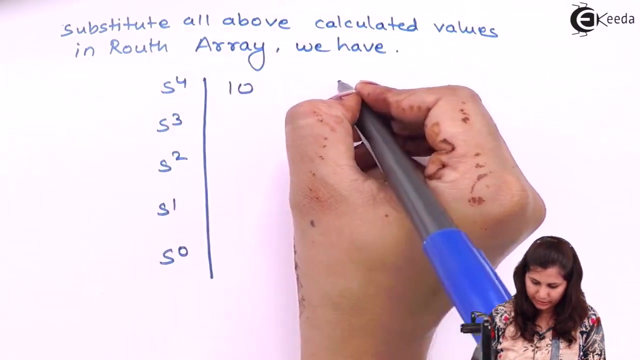 So we have calculated all the coefficients, or all the elements of the root array. So this was s to the power 4, s cube s square s1 and sz s4 was 10, 3, 9.. Then we have 9, 6, 0.. 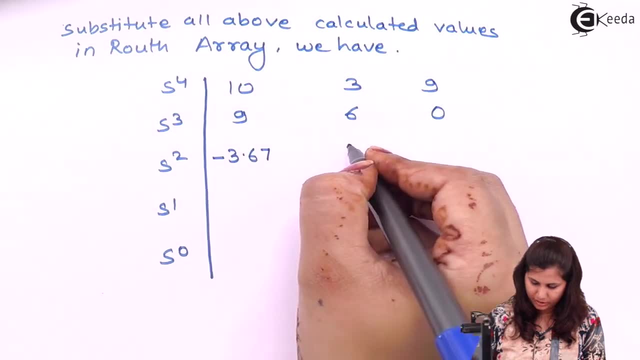 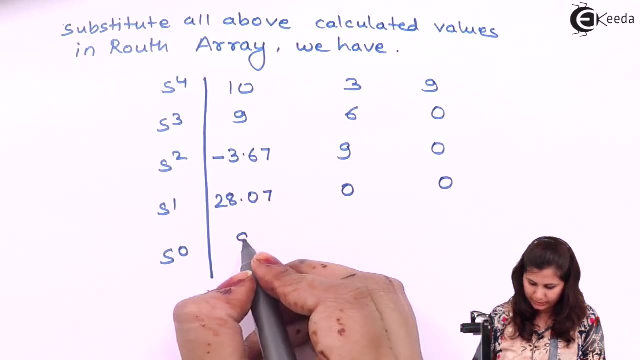 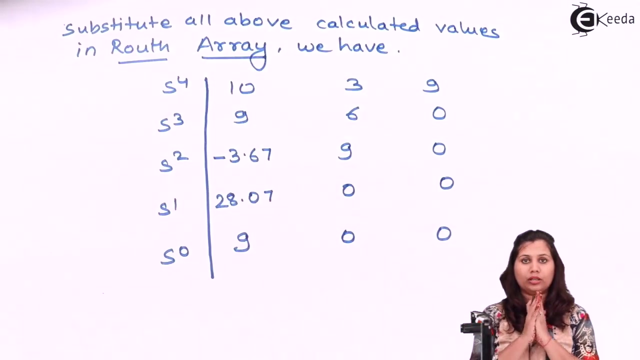 Then we are having minus 3.67, 9, 0.. This is 28.07, 0, 0, and then 9, 0, 0.. So this is what. This is the complete root array. So now, to obtain the stability, what we have to do? We have to check. 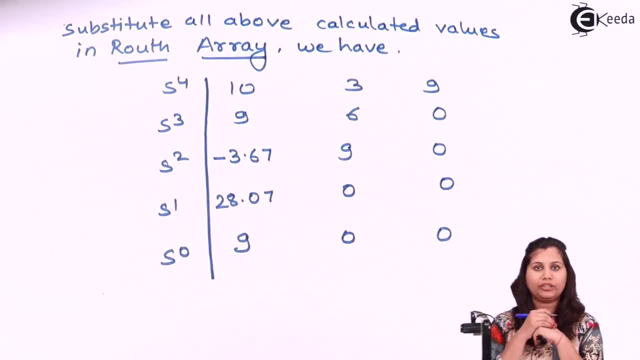 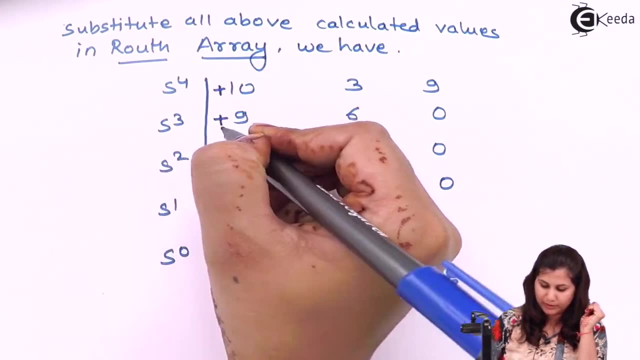 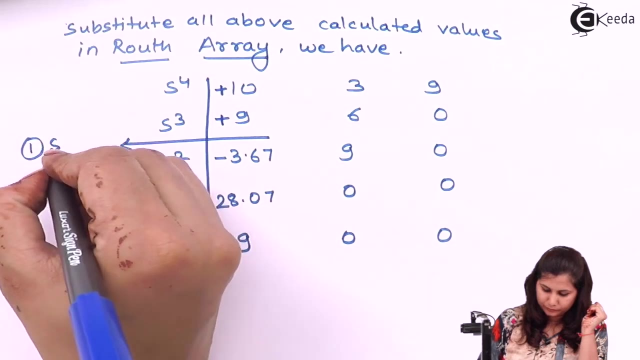 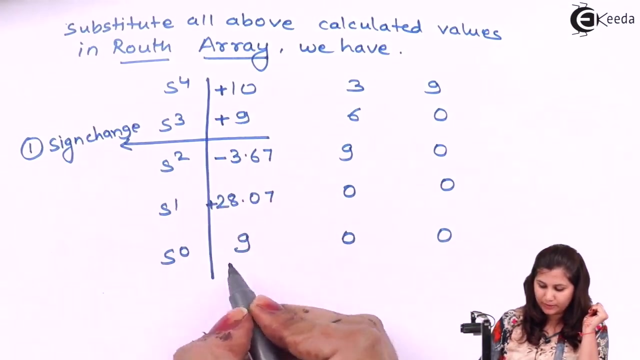 the number of sign changes in the first column of the array. This is the first column. Check the number of sign change. This is positive. this is positive. this is negative. So there is one sign change here. So this is negative. this is positive. this is positive. So, negative to positive, there is again. 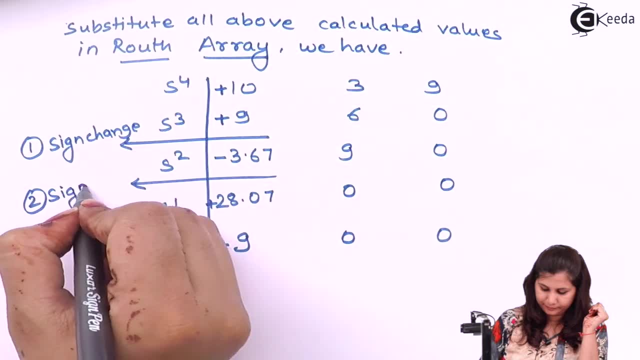 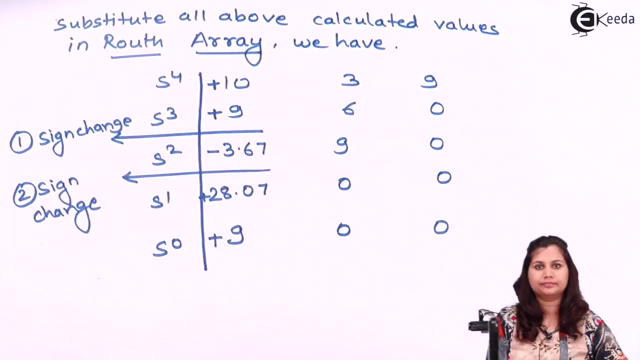 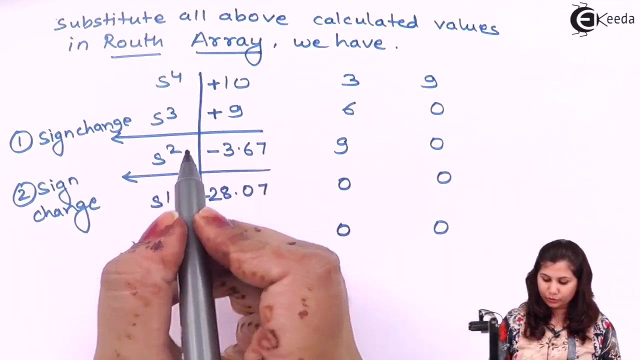 another sign change, So there are two sign changes in this first column of the array. This video is in continuation of the topic of the problem number 1 on Ruth Hurwitz criteria. So in the first column of the root array there are two sign changes, So there will be two roots which are lying on the